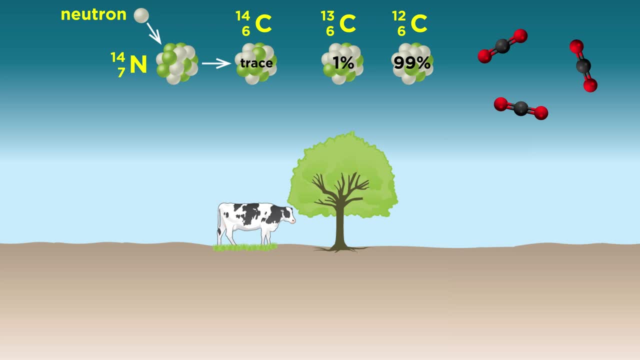 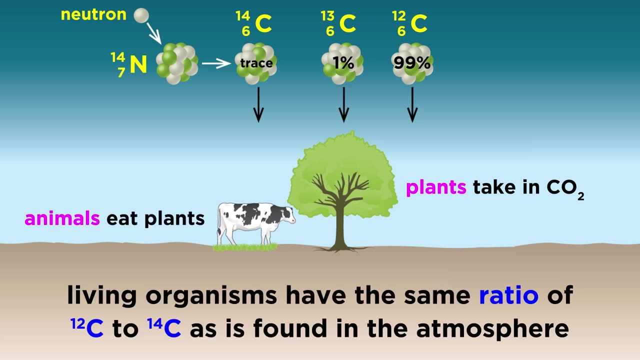 the carbon dioxide in the atmosphere. Carbon dioxide is absorbed by plants and plants are eaten by animals, so living organisms which are constantly bringing in material and expelling waste will display the same ratio of carbon-12 to carbon-14 as is found in the atmosphere. 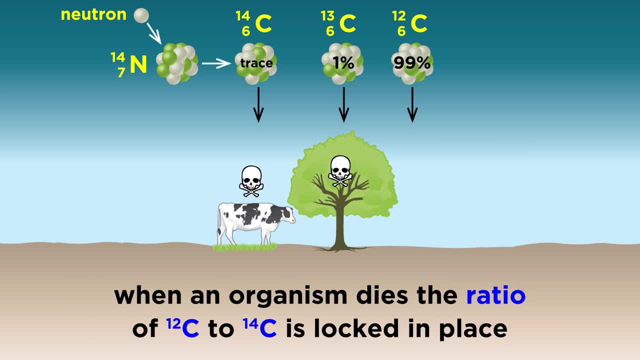 But when an organism dies and all cellular processes come to a halt, no more material will be going in or out of that organism. so no new carbon-14 can become present and all of the carbon is locked in place. Carbon-14 will then undergo beta emission to become nitrogen-14 again, thus gradually, 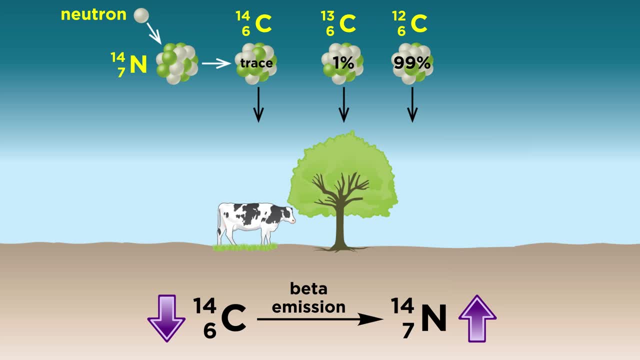 decreasing the amount of carbon-14 in the organism, And this process displays a half-life of 5,730 years. That means that if we find a wooden artifact made from a once-living tree and then use a mass spectrometer to determine that the ratio of carbon-14 to carbon-12 in that artifact 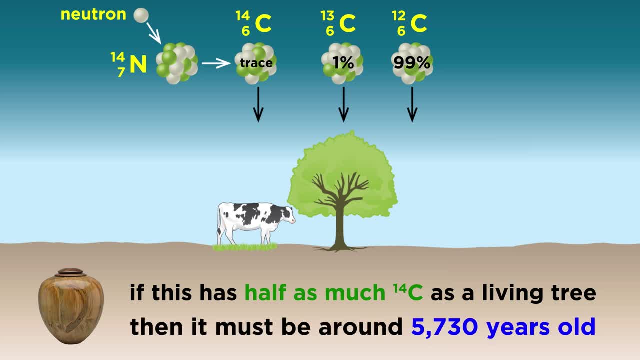 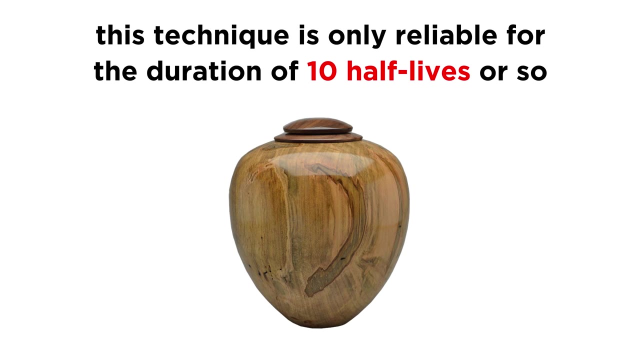 is half of what it is in a currently living tree. that object must be around 5,730 years old, because half of the carbon-14 present when the wood was part of the living tree has already decayed. Of course, if any more than ten or so half-lives have elapsed, this technique becomes less. 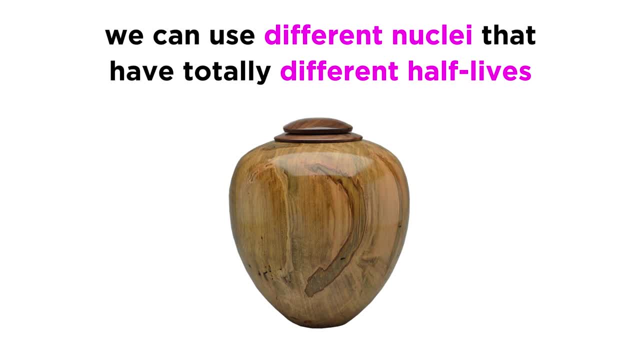 and less reliable. However, there are many other radioactive nuclei that we can use that have totally different half-lives and thus allow us to date objects of a wide variety of ages: Potassium, argon, lead. these all have radioactive isotopes that can be examined if an object 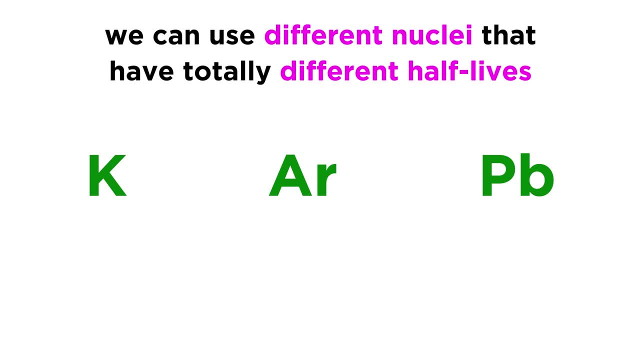 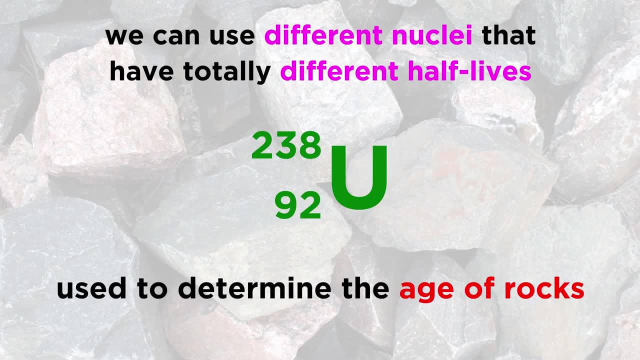 in question contains appreciable amounts of that element, and many of these allow us to date objects much older than 50,000 years: Uranium-238.. Uranium-238 is commonly used to determine the age of certain rocks, including the oldest. 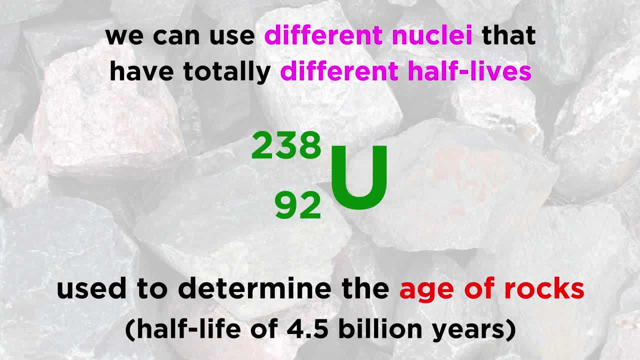 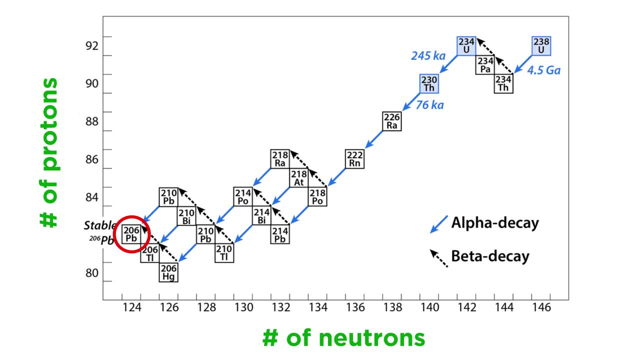 rocks on earth, since this particular nuclide has a half-life of 4.5 billion years. Uranium-238 undergoes a decay series to produce lead-206, so we simply measure the ratio of uranium-238 to lead-206 in a rock to get its age. 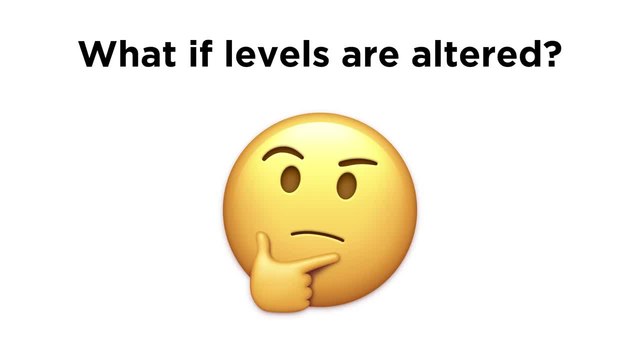 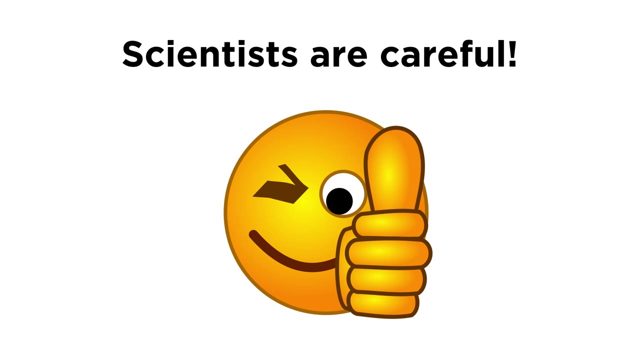 There are those who question the accuracy of such methods, And indeed there must be confidence that an object has not had its levels of these nuclei altered over time somehow in order to trust the results of these techniques. But scientists are not naive. They know how to be rigorously empirical. 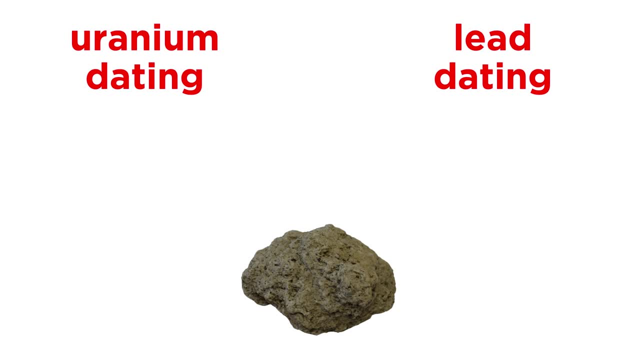 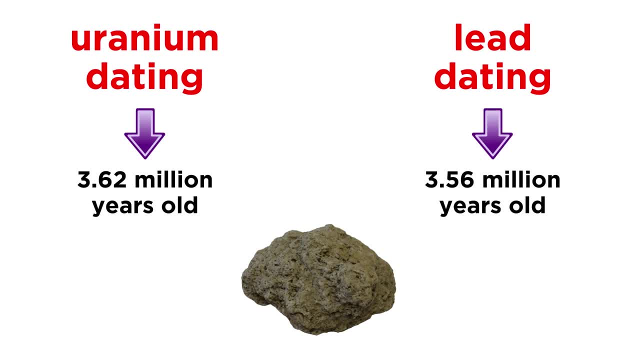 Uranium-238.. And then lead dating is used to find that the same rock is 3.56 million years old. it is extremely unlikely that the rock is not approximately that age, because these are totally disparate materials and the agreement of these measurements corroborates the age of the rock. 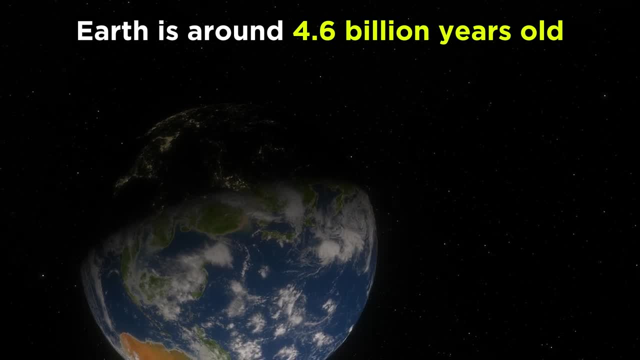 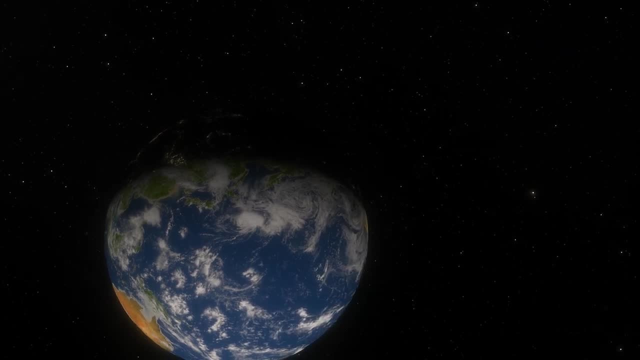 used to determine the approximate age of the Earth, which is around 4.6 billion years old. This is a value which is around 4.6 billion years old. This is a value that reinvents when ourselves home. that home really puts our existence into perspective and truly demonstrates the power of science. 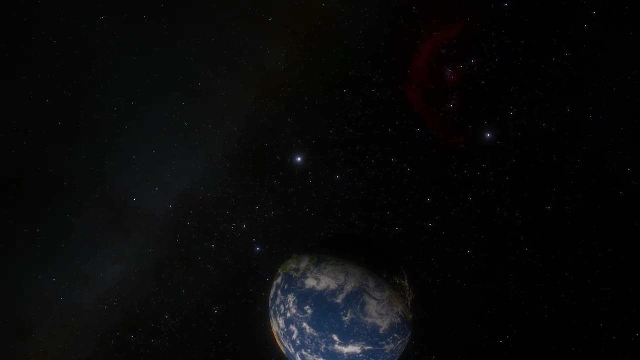 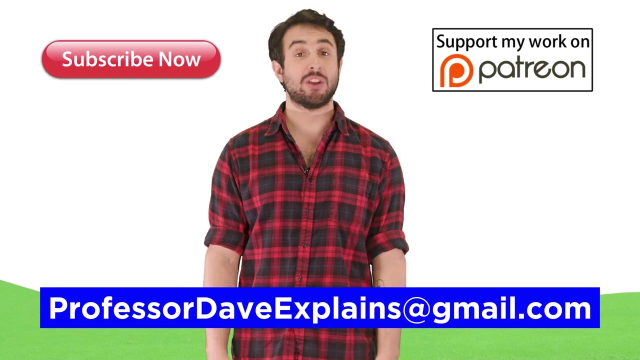 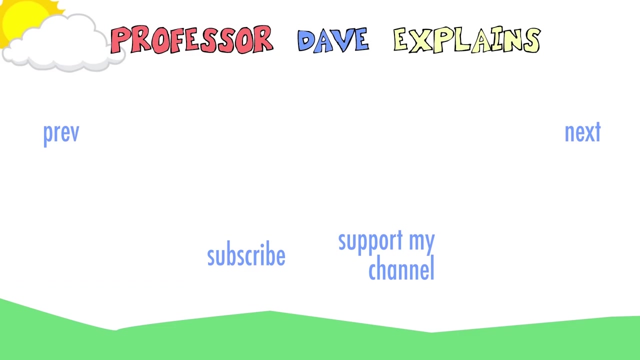 in helping us understand the universe. ©. transcript: Emily Beynon. 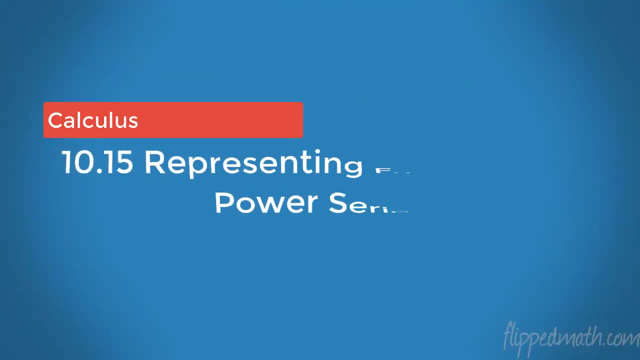 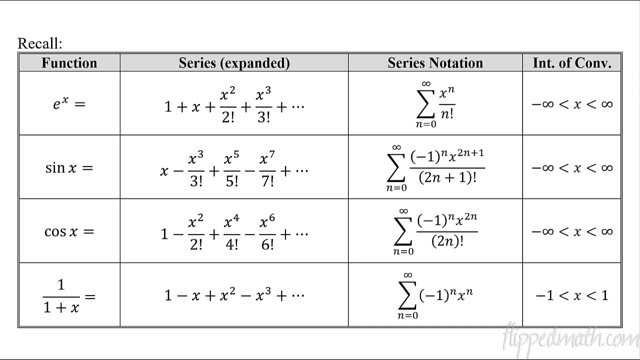 Hello Cal kids, Welcome back to another lesson in calculus. This is Mr Bean, and today we're going to do our last lesson of calculus. This is so exciting. I'm happy for you. I'm really happy for me, because this has been a couple years of making calculus videos and this is it. This is.